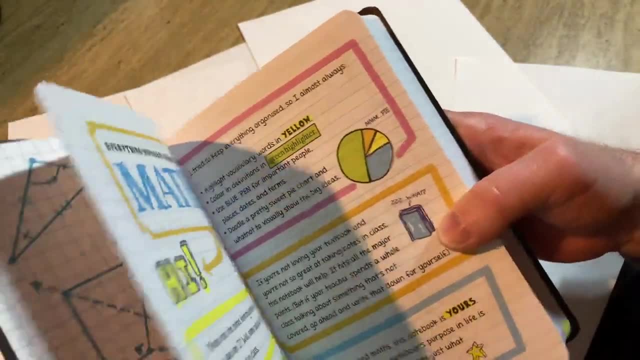 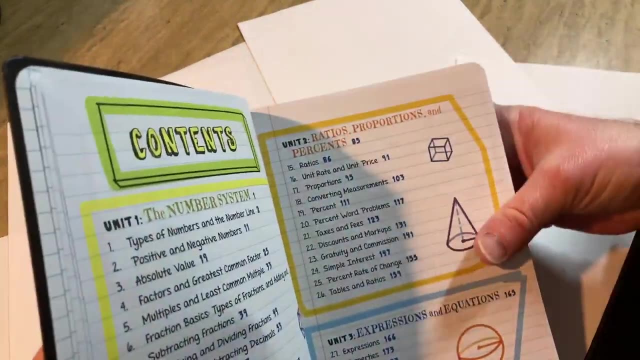 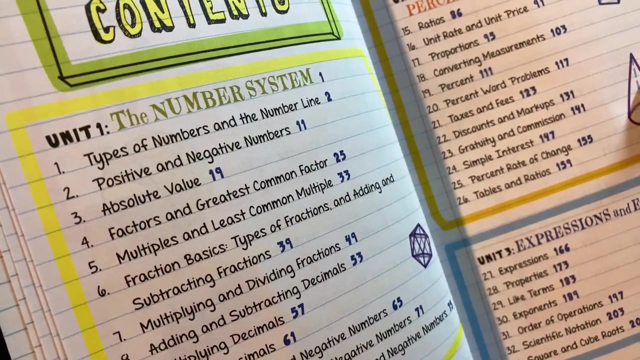 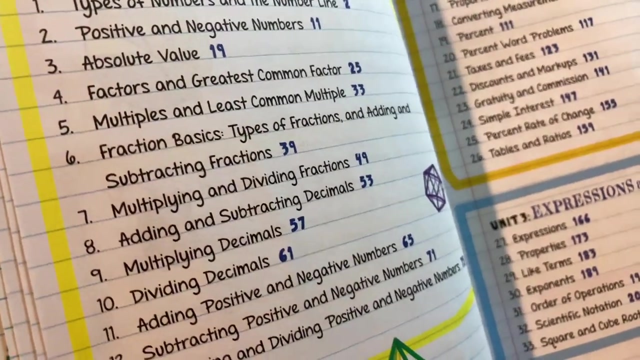 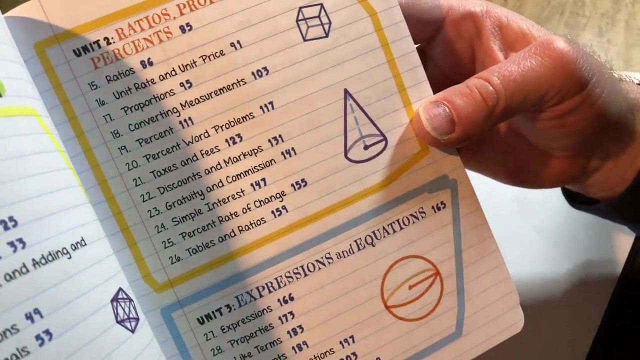 But you can use this book for self study. It's really intended for that purpose. Let me show you some of the contents And you'll see that it really really starts from the beginning. So it starts with numbers, the number system, types of numbers and the number line, positive and negative numbers, absolute value factors and greatest common factor, multiples and least common multiples- really basic stuff- and ratios, proportions and percents expressions. 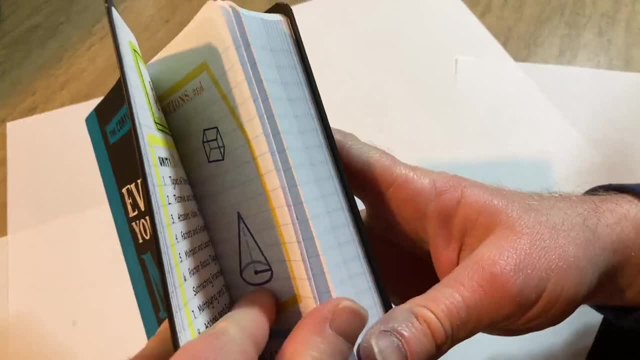 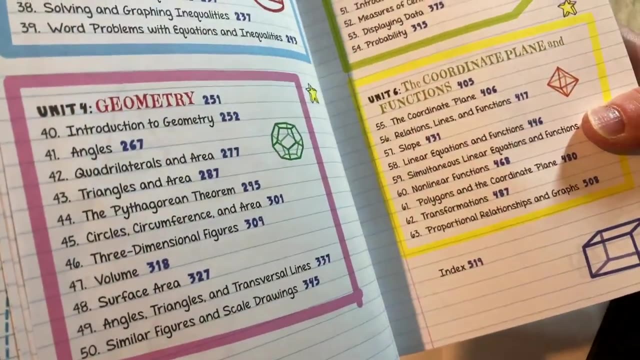 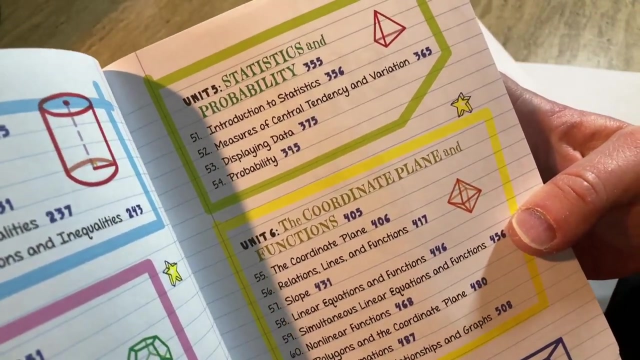 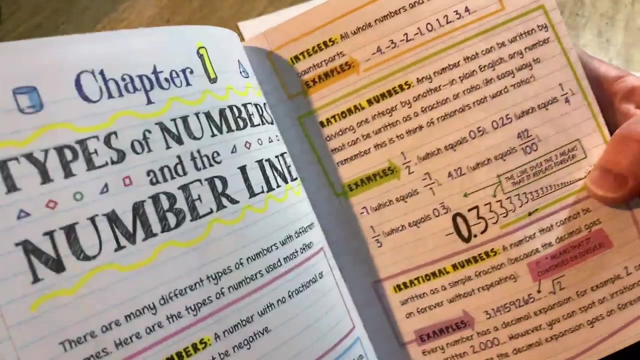 and equations. Let's turn the page. Geometry. So it also has geometry in it. So maybe your geometry is rusty. This is a nice way to bring it back up to speed. It even has statistics and probability, And then the coordinate plane and functions. Let me just show you how it starts really quickly, so you can see how basic it actually is. There are many different types of numbers with different names. Here are the types of numbers used. 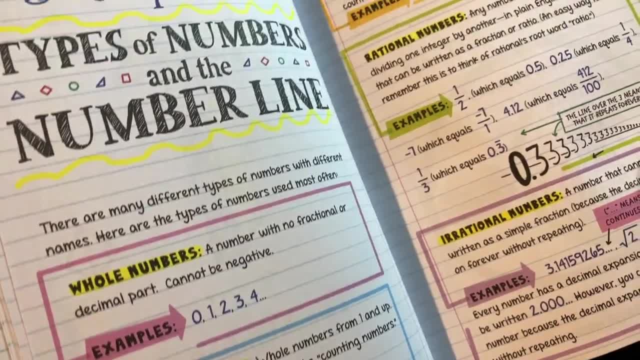 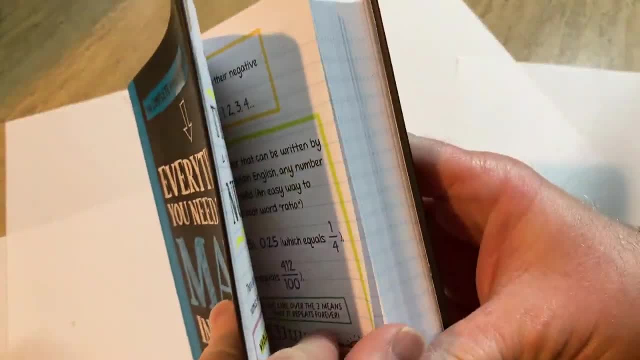 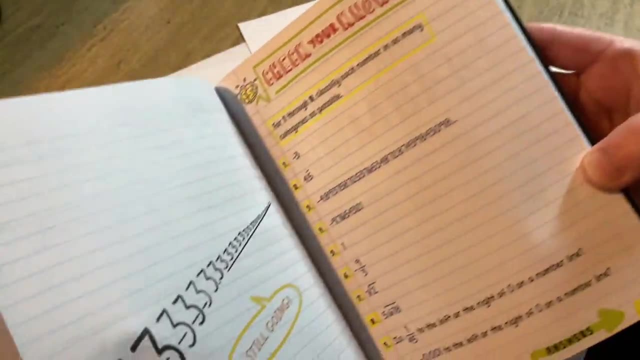 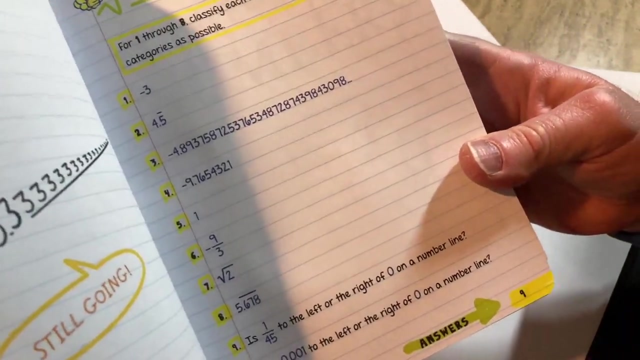 Most often talks about the whole numbers, the natural numbers, integers, rational numbers, irrational numbers- And it's a fun book. You know it's a really fun book because it just has fun stuff in it. You know the type setting- I mean still going right, Really really fun. It also has exercises And then when you do the exercises you can turn the page and you get the answers. 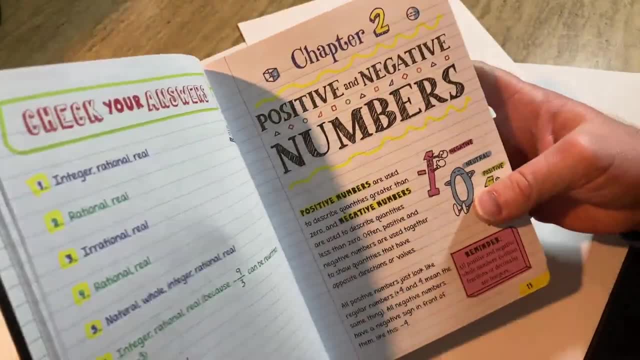 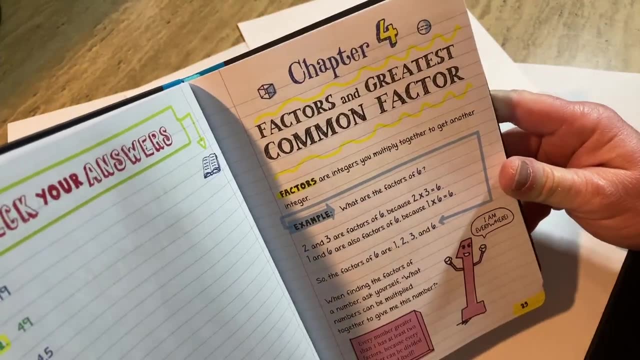 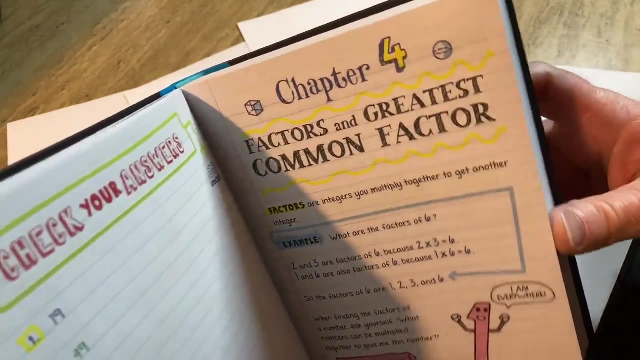 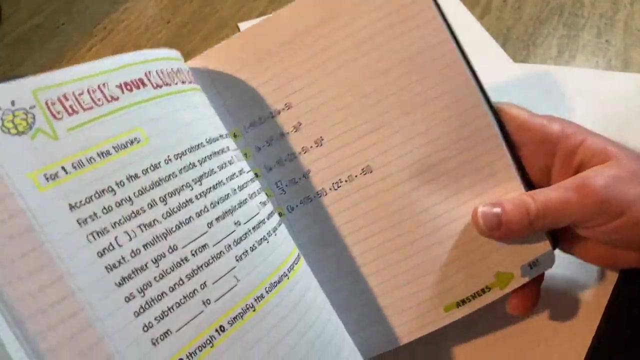 All right, It gives you the answers, So perfect for someone who has been out of school for a long time and just doesn't know a lot of math. Now, if you already know some math, then this is probably not the book for you. Now, I'm not saying that you can't learn from this book. I mean it does have a lot of topics. It has some statistics and probability. It's got some geometry, So this book probably has something you don't know. But if you already know some math then it's probably not worth getting into. 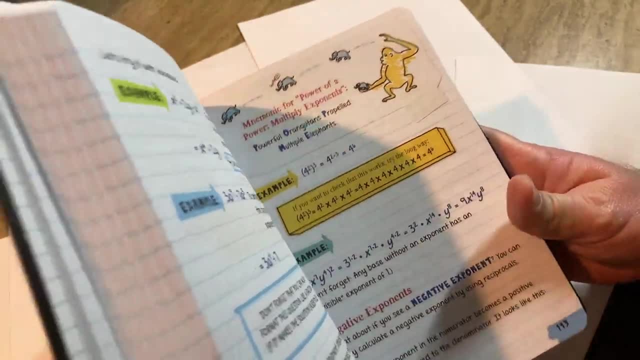 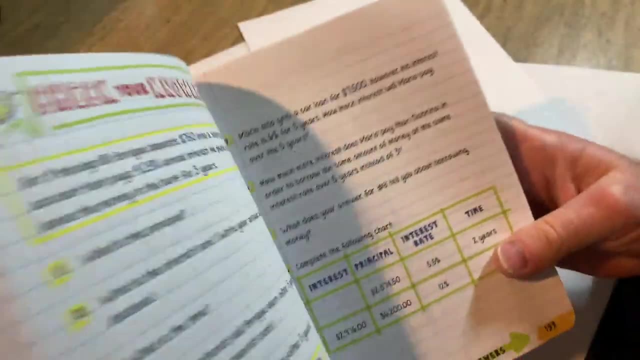 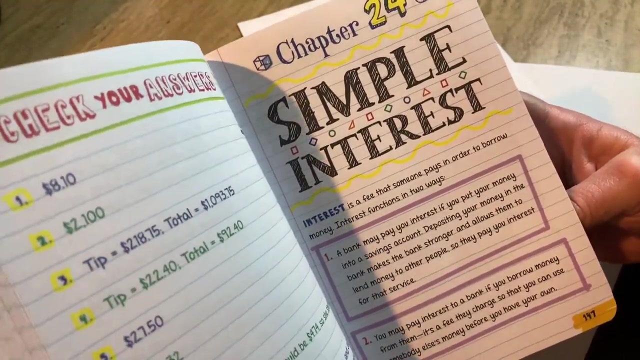 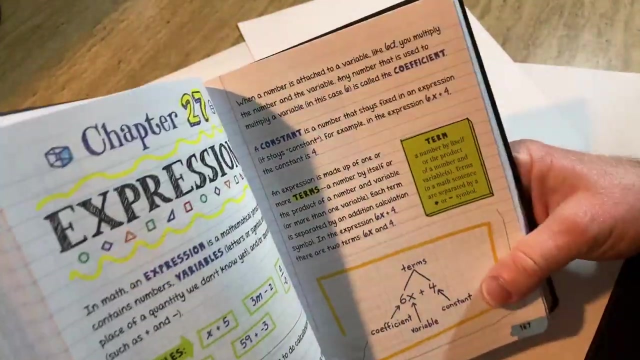 I bought this book because I collect math books and I try to have at least one copy of every math book out there- And there's a lot of math books. That's why I have so many books, because I collect them. I want to have all of them: old ones, new ones, different editions. I'm a pretty serious collector. Let's look at some of the sections in this book so you can see what it's like. Here it talks about expressions In math. an expression is a mathematical phrase that contains numbers. 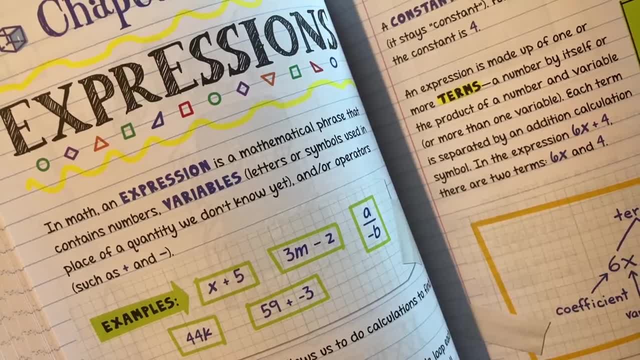 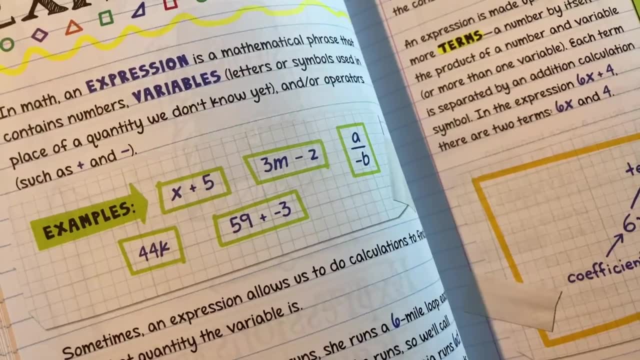 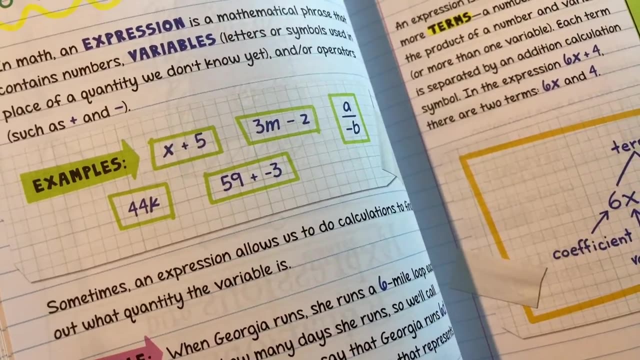 Variables, letters or symbols used in place of a quantity we don't know yet, and or operators such as plus and minus. So here we see examples: x plus 5, 3m minus 2, a over negative b, 44k, 59 plus negative 3.. Sometimes an expression allows us to do calculations to find out what quantity of variable is. 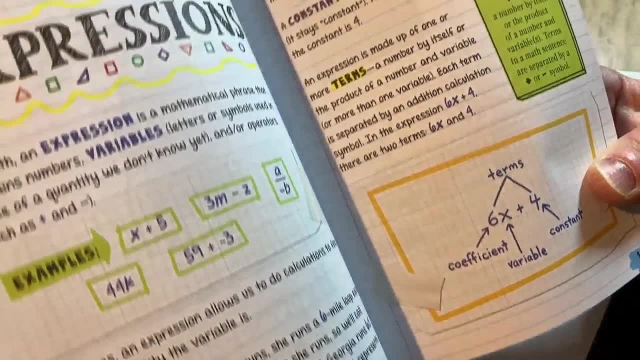 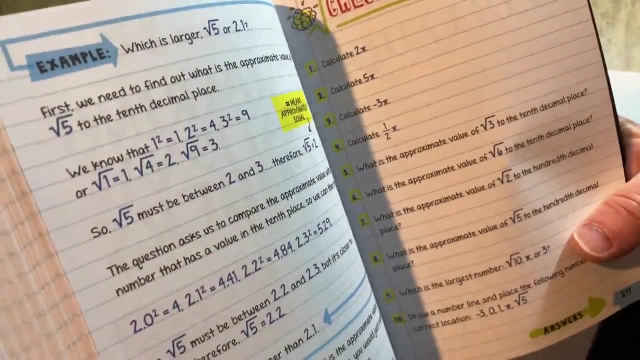 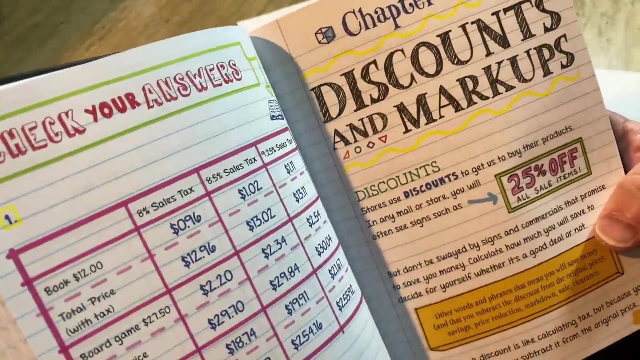 Then here it gives you an example so you can learn, And it's an interesting book. I always wonder, like, who wrote this book, Because it's published by Workman Publishing but like no author is given, I'm assuming it's like a team of people that work on this book. It's just really well done and it's really fun. 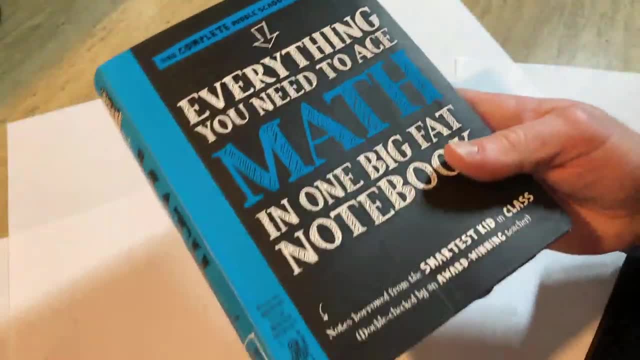 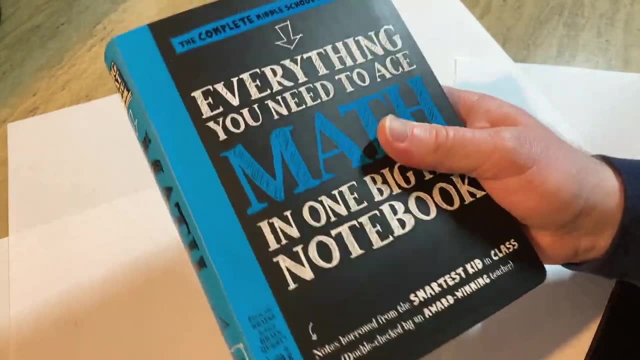 Another thing about this book I should mention- and this is true for all of the books published by Workman Publishing, at least the ones I have, I have almost all of them- is that it's a soft cover, but it's a weird type of soft cover. 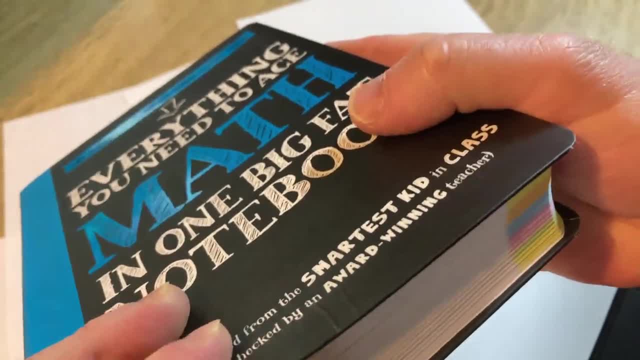 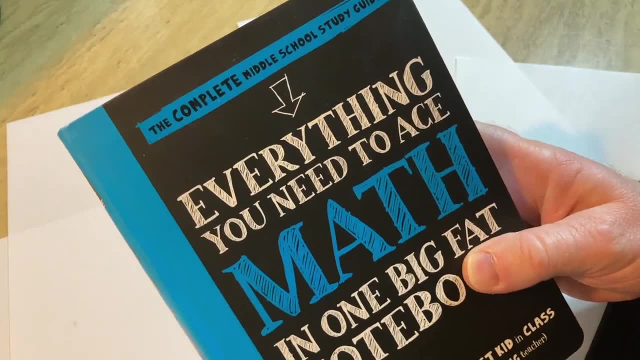 Like the material. it's not like the regular soft covers. It just seems like it's a soft cover. It just seems like it's almost like a hard plastic but it's bendable, which I guess is intentional because it is intended for middle school students. 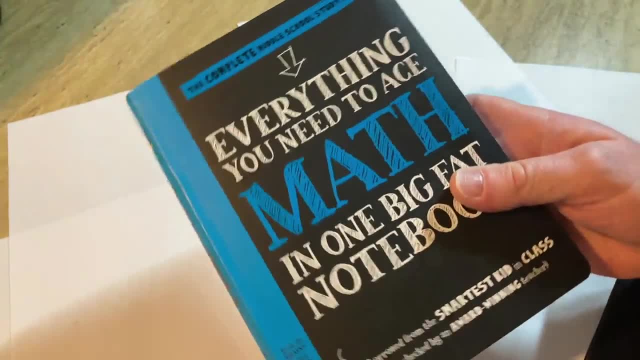 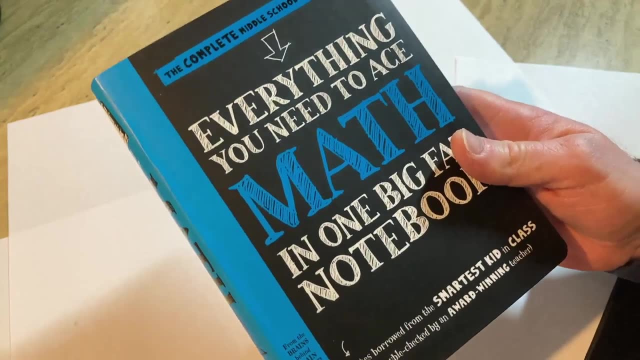 And so I guess the you know the stereotype is: oh you know, kids will be kids. Maybe people will throw the book around. I haven't tested the quality of the book, I have not decided to take this book or any of my other books published by this company, and I haven't, you know, thrown them around and tested them. 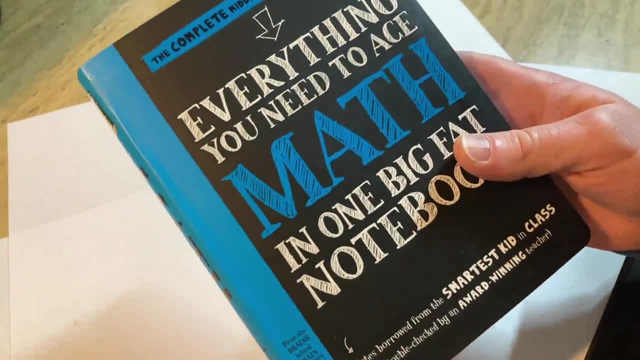 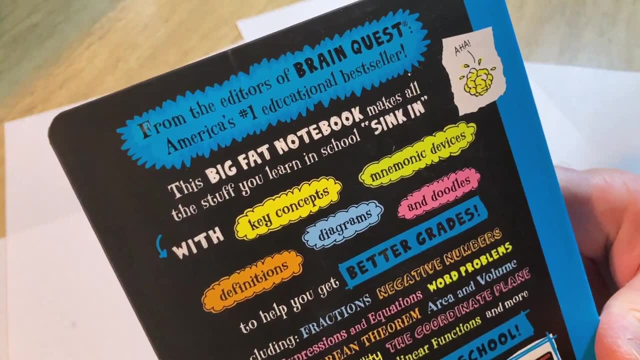 But it feels like. it feels like it would hold up really, really well to some abuse. Here's the back of the book, says from the editors of BrainQuest, America's number one educational bestseller. the big fat notebook makes all the stuff you learn in school sink in. 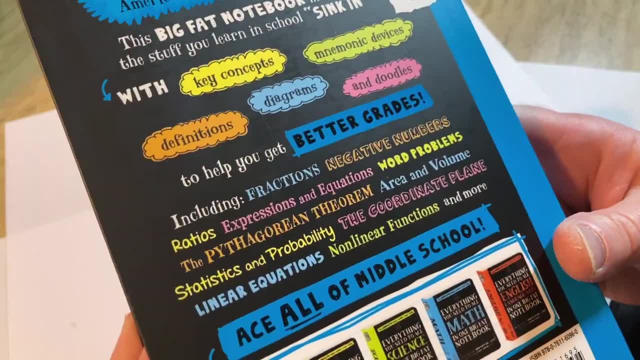 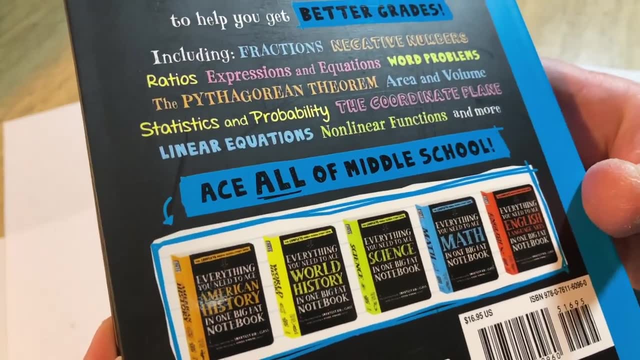 Yeah, Yeah. So it's intended to, you know, help you do better in school. I'm looking at this from a self-study perspective. You know, maybe you're an adult and you didn't finish high school, or you barely even went to high school, or you just forgot everything. 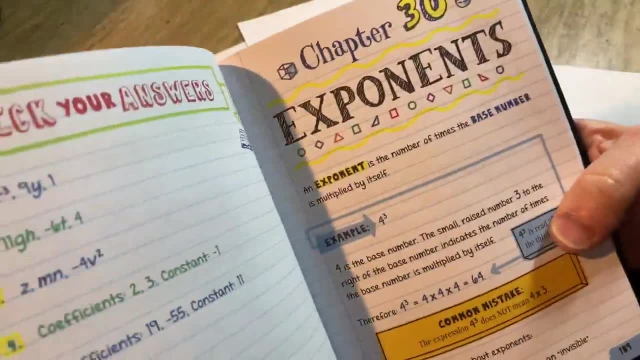 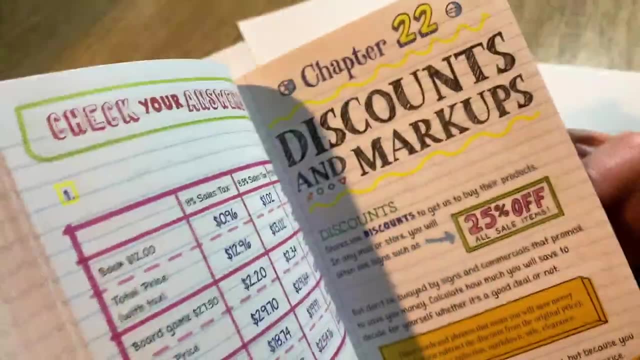 You can get a book like this one And you can get started with mathematics right away from the very beginning. At the same time, if you, if you already know some math, then there's better choices, right There's. you can get an actual textbook. 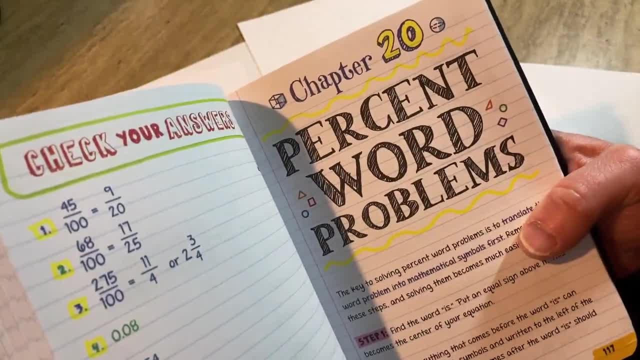 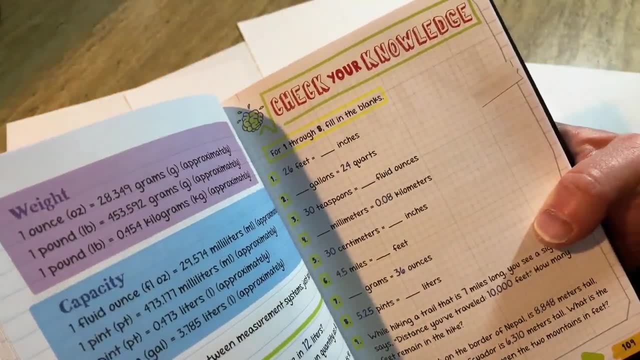 For example, if you already know some math and you're looking to jump into calculus, you'd probably be better off getting like a college algebra textbook, like the one by Blitz, or College Algebra Essentials, which is an actual college level textbook that has considerable 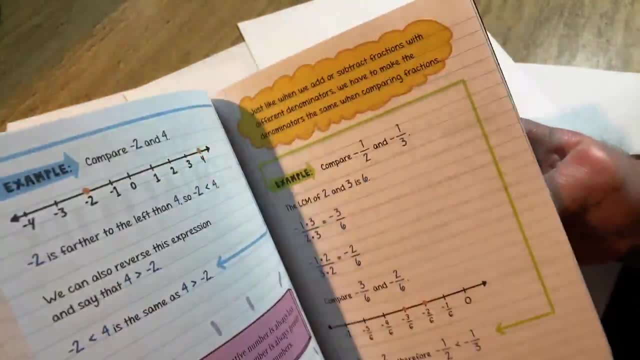 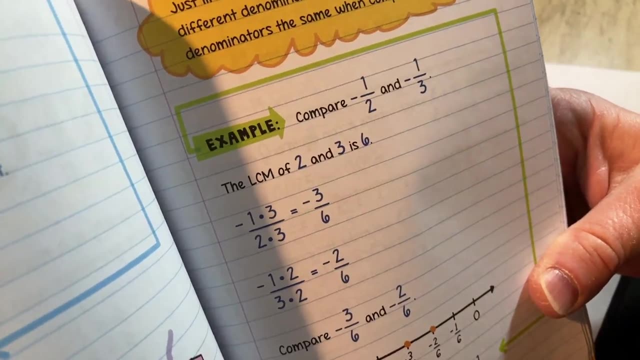 More math in this. This is perfect for someone again who just doesn't know, doesn't know a lot of math. Here's an example. Compare negative one half and negative one third. The LCM that's called, the least common multiple of two and three is six. 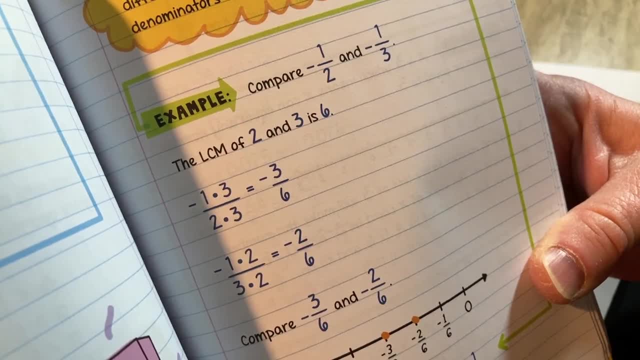 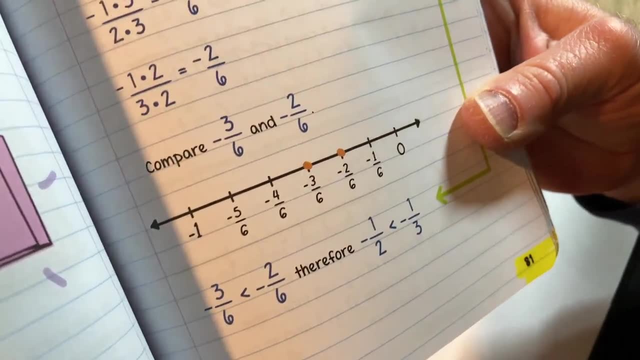 Cool, And then so you basically Write them with the same denominator and then you can compare them Like this on a number line. Pretty cool, right? So it shows you stuff That you know. you might not know even if you, if you think you know math. 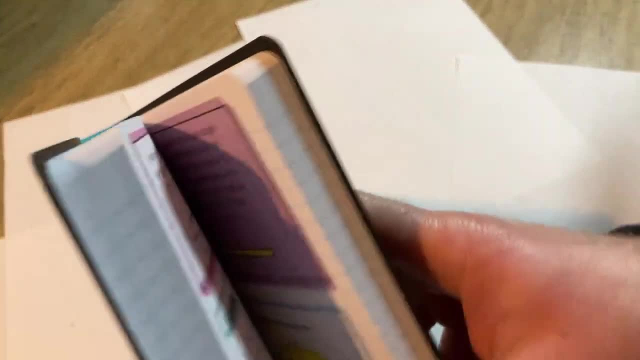 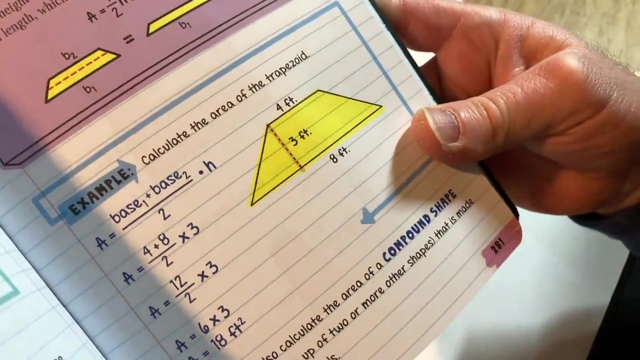 And as always I will. I'll try to leave a link. I'll try to remember to leave a link in the description of this video so you can check it out if you want to. It shouldn't be too expensive. That's another thing about these books. 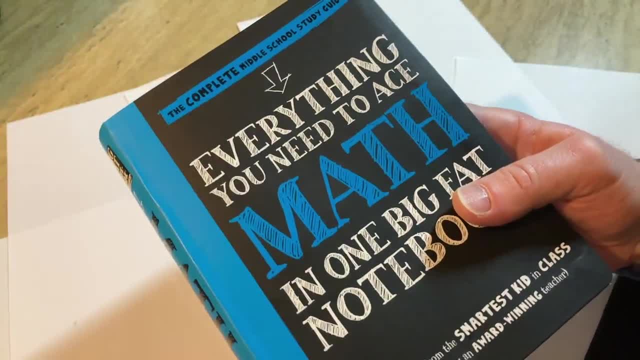 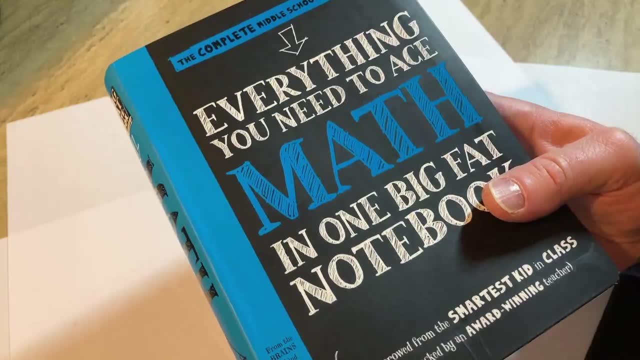 All of these books by this company. they're all really inexpensive, Like if you compare the price of this to the price of a textbook, it's it's ridiculous, right? This? This is so much cheaper than an actual textbook. But you know, it's not the same, not the same. 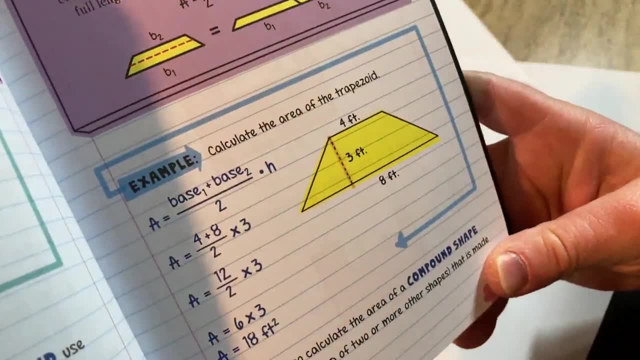 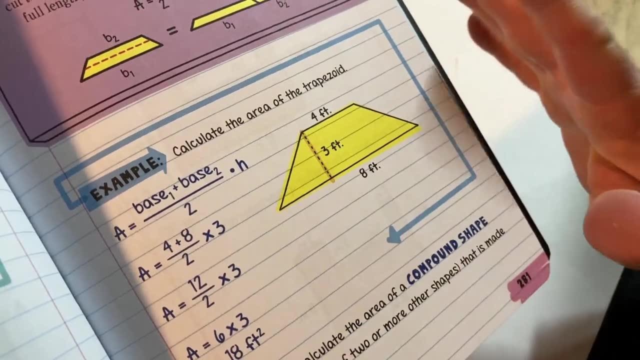 This is interesting because I was I was doing some math for my other YouTube channel, Epic Algebra. I have another channel- It's called Epic Algebra, where I just post like algebra content and like really basic math content and some harder stuff to just to mix.